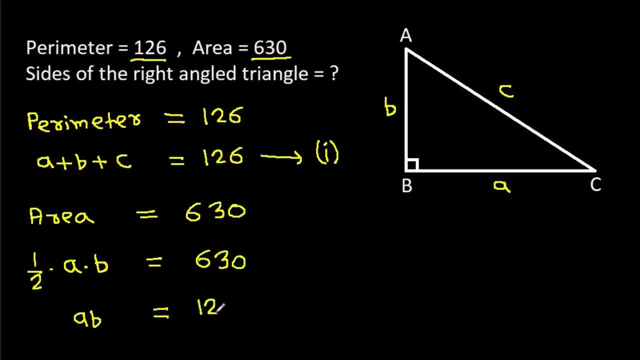 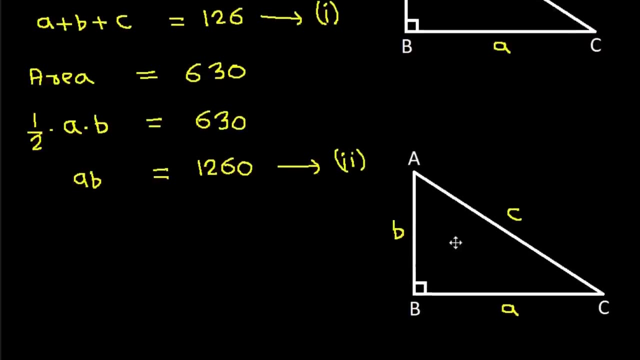 So AB, it will be 260.. Suppose it is equation 2. and now by Pythagoras theorem we can get A squared, P plus B squared is equal to C squared. Suppose it is equation 3.. So we have A, P plus B, C is 126. it is equation 1.. 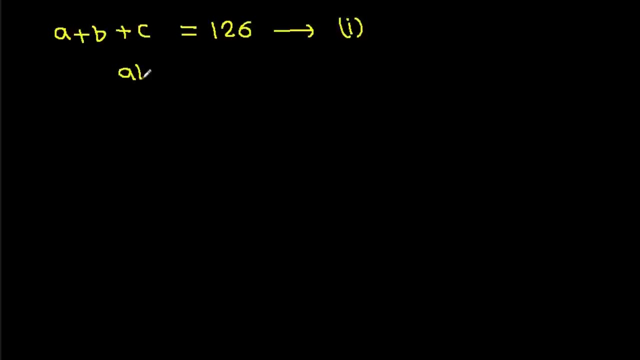 AB is 126 and P plus B is a equation 3 and it is a line. P be a line and P must be a line. A is equal to 3 in perimeter and area is 226.. 760.. It is equation 2.. And a square plus b square is c square. It is equation 3.. And 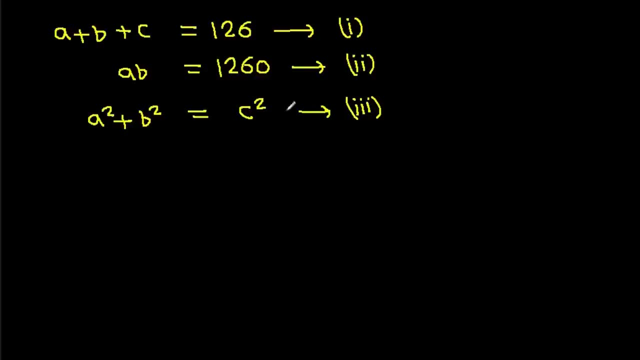 now from equation 1, we have a plus b plus c is 126.. And a plus b it will be 126 minus c, And if we square it both sides then it will be a square plus b square Panas b square Panas 2ab is equal to 126 square Panas c square minus 2 times 126 times c. 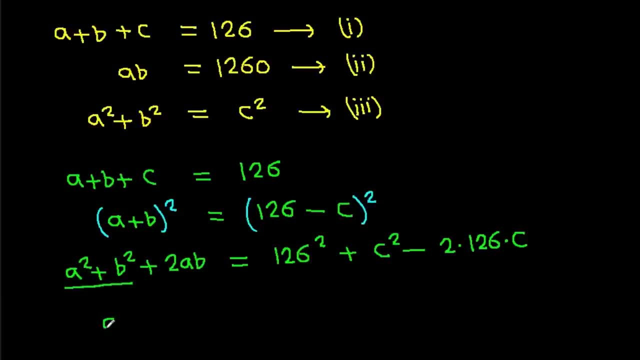 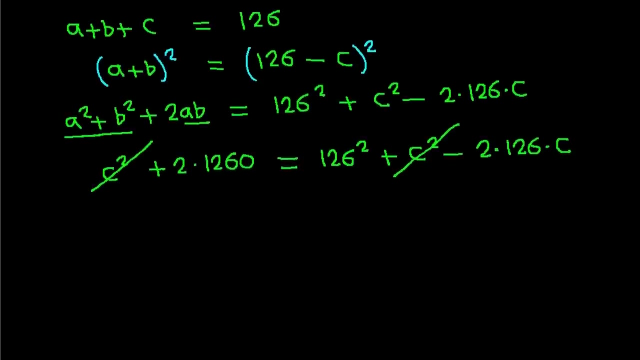 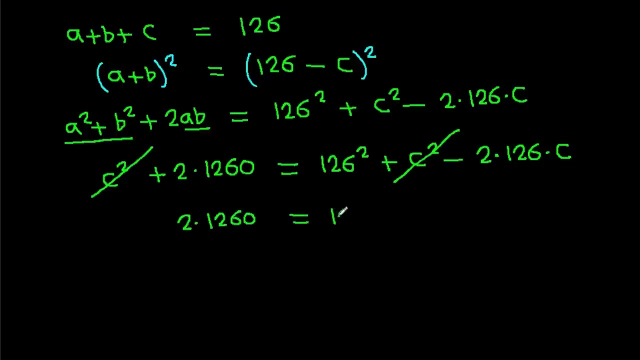 And a square Panas b square, it is c square Panas 2 times ab is 1260.. It is equal to 126 square Panas c square minus 2 times 126 times c, And c square will get cancelled. So 2 times 1260 it is equal to 126 square Panas 2 times 126 times c. 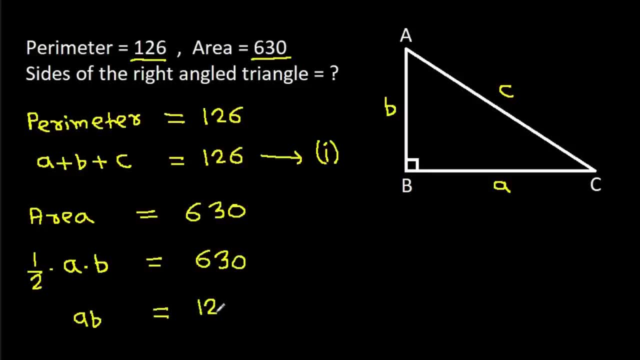 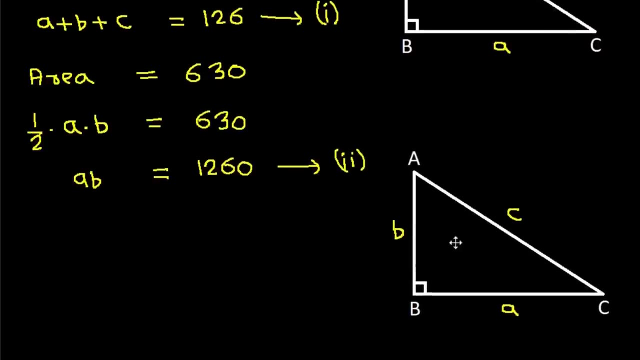 So AB, it will be 260.. Suppose it is equation 2. and now by Pythagoras theorem we can get: a square plus b squared is equal to c squared. Suppose it is equation 3.. So we have A plus b plus c is 126.. It is equation 1.. 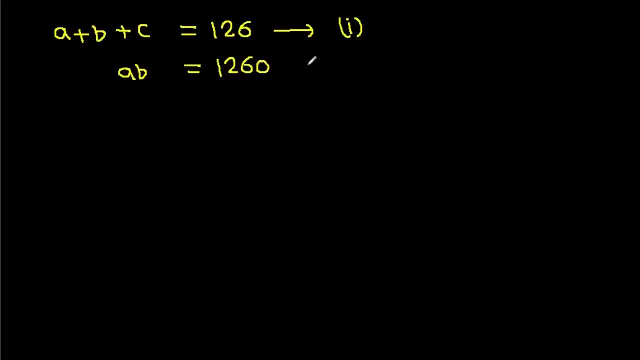 AB is 263.. it is equation 2, and a square plus b square is c square. it is equation 3.. And now from equation 1, we have a plus b plus c is 126 and a plus b it will be 126. 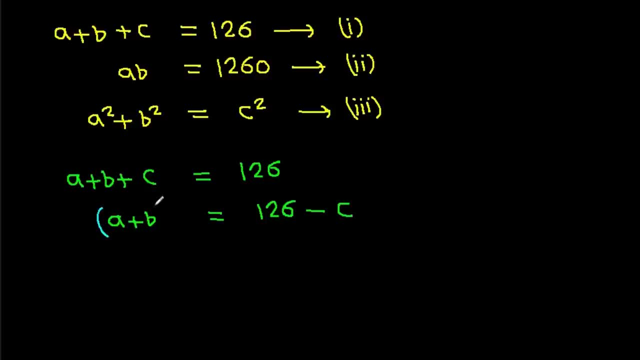 minus c And if we escape it both side, then it will be a square plus b square is 126 and c square is 126.. is equal to 126 sqe plus c sqe minus 2 times 126 times c and a sqe plus b sqe, it is c? sqe. 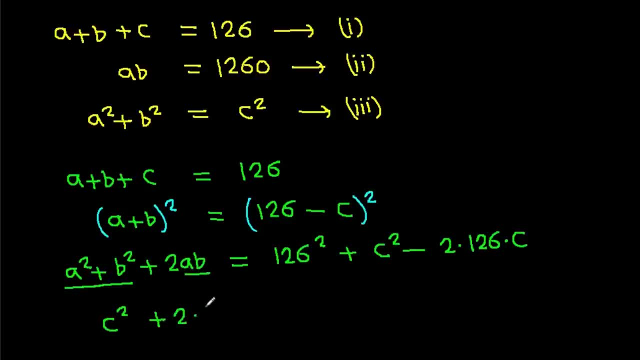 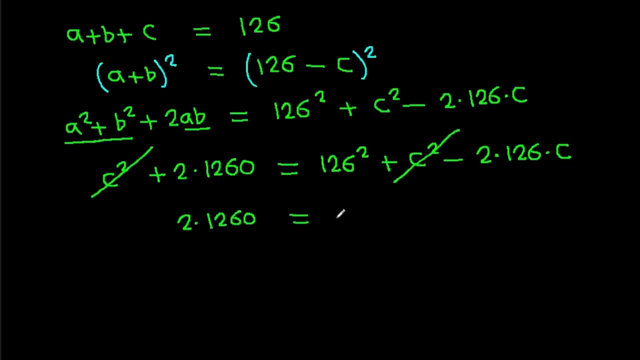 plus 2 times ab is 1260. it is equal to 126 sqe plus c sqe minus 2 times 126 times c, and c sqe will get cancelled, So 2 times 1260.. 1260: it is equal to 126 sqe minus 2 times 126 times c, and it is 2 times 1260, it is 126. 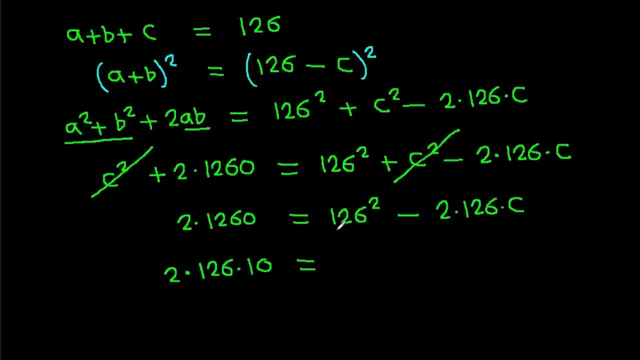 times 10.. It is equal to 126 sqe. It is 126 sqe. It is equal to 126 times 126, minus 2 times 126 times c, and 126 will get cancelled. So it is 2 times 10: is equal to 126 minus 2 times c. 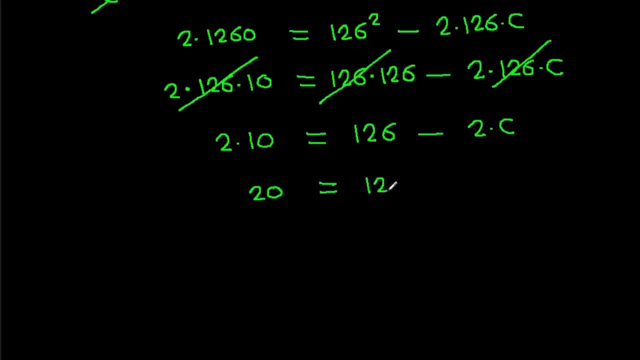 And it is. 20 is equal to 126 minus 2 times c. So 2 times c it will be equal to 106, and c will be equal to 106 by 2. So c is equal to 53.. And, And, And. 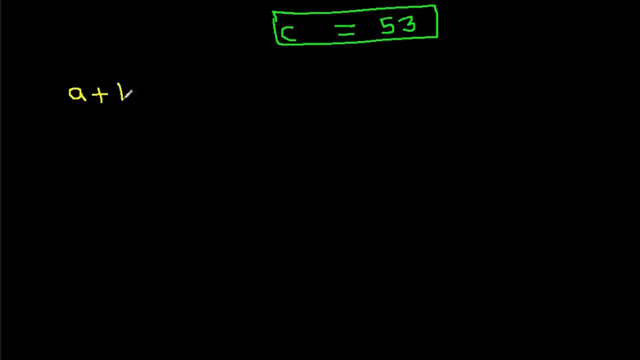 Now we have a plus b plus c is 126, and it is a plus b plus c is 53, it is 126.. So a plus b, it will be equal to 126 minus 53. So a plus b, It will be equal to 126 minus 53.. 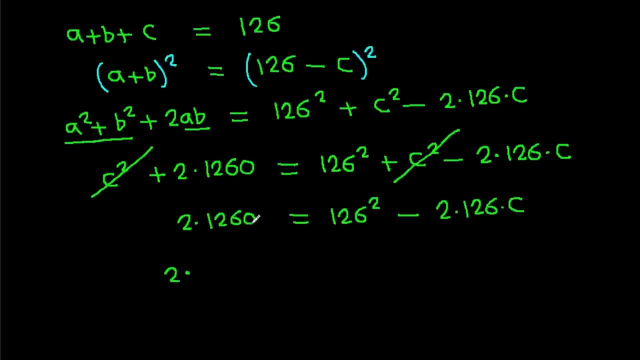 And it is 2 times 1260. it is 126 times 10.. It is equal to 1260 square Panas 2 times 126 times c. It is equal to 1260 square Panas 2 times 126 times c. 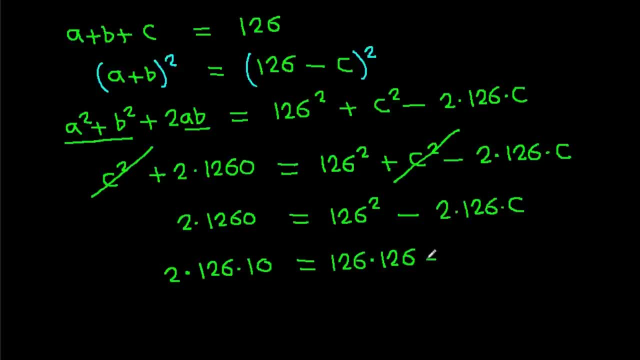 You can see that Panas is lower level than 1260 square Panas 2.. QVB is the same way because it is higher level. It is 1260 square Panas x 126.. The D times x 126.. QVB is the opposite. 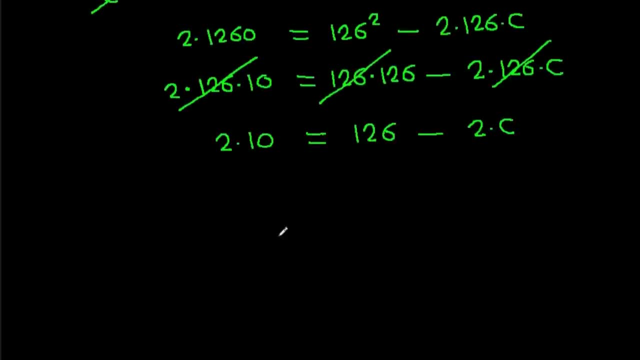 It is 126 times 126 times c. You can see that Panas, 2 times 1260 times 10 is equal to 126 times 126 times c. c and it is 20 is equal to 126 minus 2c. So 2c it will be equal to 106 and c will be. 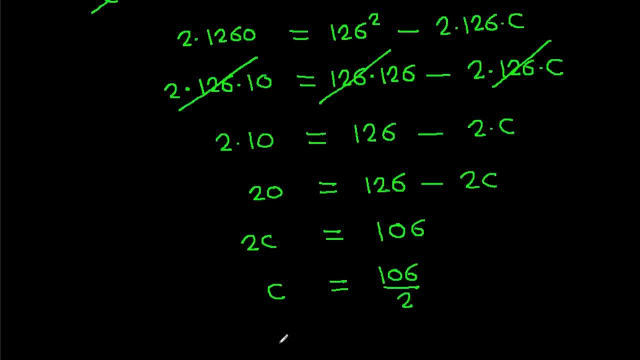 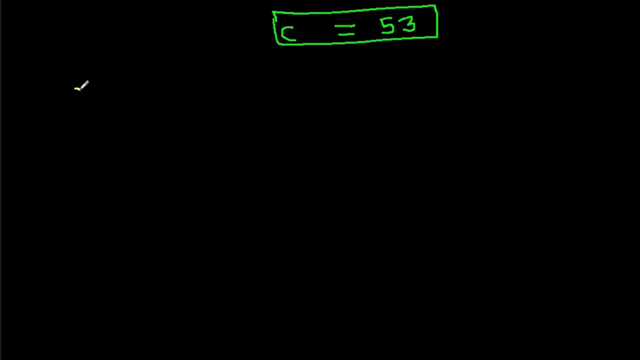 equal to 106 by 2. So c is equal to 53. and now we have a plus b plus c is 126, and it is a plus b plus c is 53. It is 126.. So a plus b, it will be equal to 126 minus 53. So a plus b, it will be equal to 73, and we 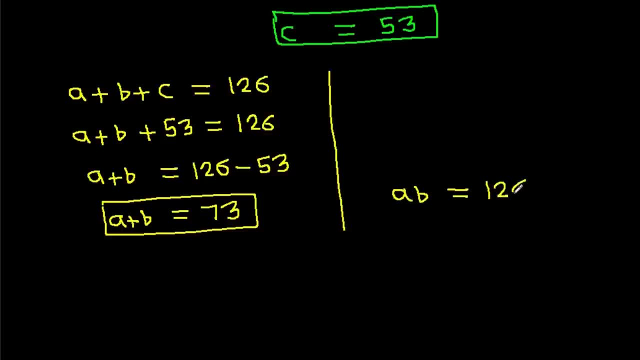 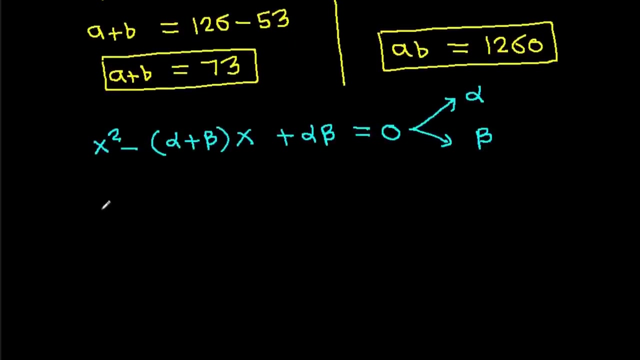 have a, b is 1260.. And for equation x square minus alpha plus beta, x plus alpha beta is equal to 0.. The root of this equation is alpha and beta. So for equation x square minus a plus b, it will be equal to 0.. So a plus b is equal to 0.. So a. 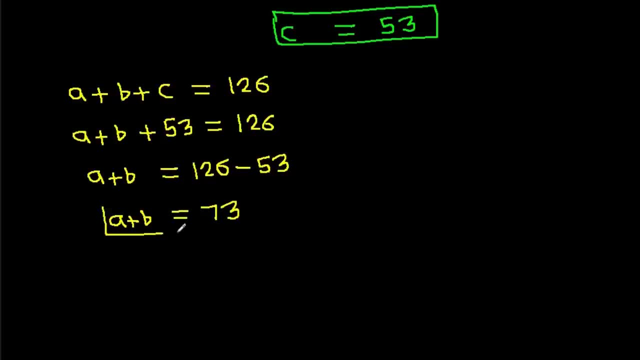 Therefore it will be equal to 73. Then we have: Therefore it will be equal to 73. And we have. So b is 1260 at c. It is a plus a. Either it is greater than, greater than greater than or equal to c. 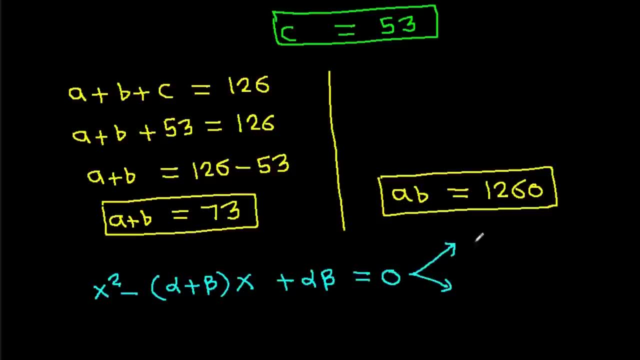 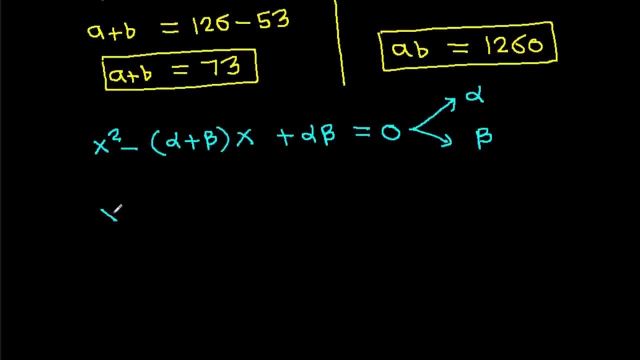 to zero. the root of this equation is alpha and beta. So for equation x square minus a plus b, x plus ab is equal to zero. the root of this equation will be a and b, And it is: x square minus a plus b is 73,. x plus ab is 1260, it is equal to zero. 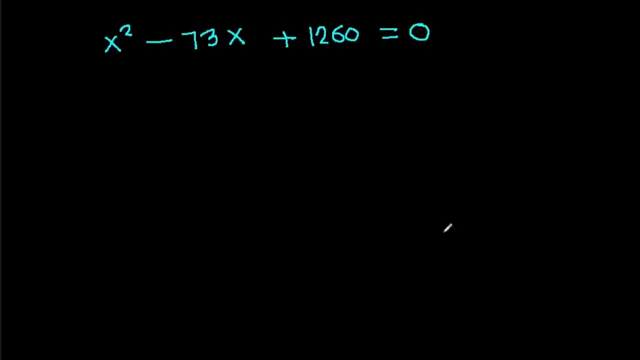 And now 1260, it is two times 1260, it is two times 1260, it is two times six hundred thirty, two times three hundred fifteen, three times one hundred five, three times thirty five and five times seven. 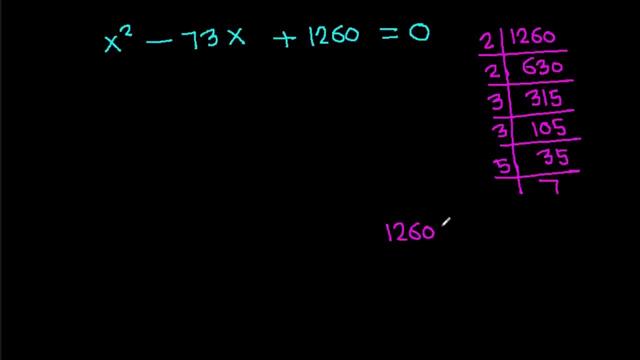 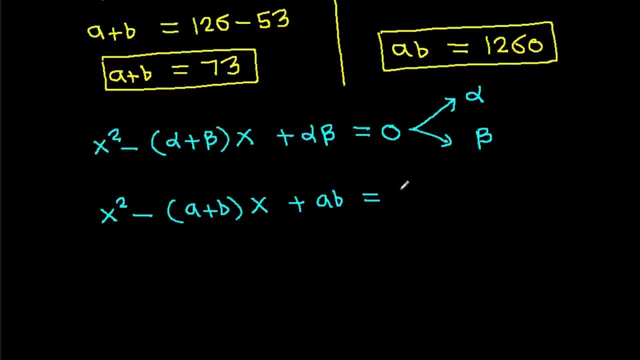 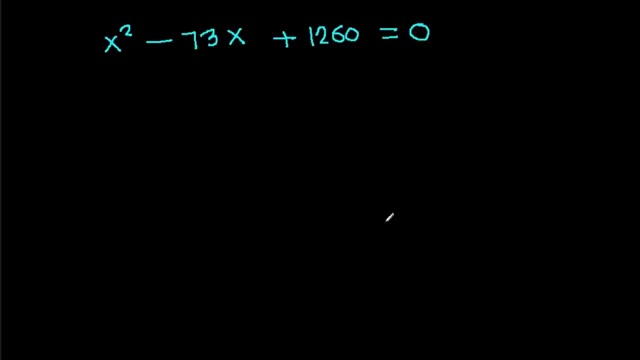 x plus ab is equal to 0.. The root of this equation will be a and b, And it is x square minus a plus b is 73x plus ab is 1260.. It is equal to 0.. And now 1260, it is 2 times 630.. 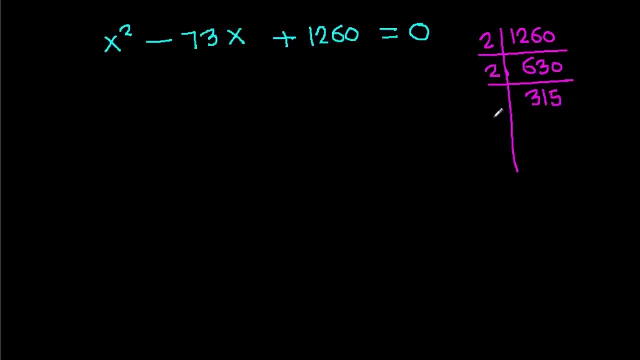 2 times 315.. 3 times 105.. 3 times 35.. And 5 times 7.. So 1260.. It is 2 times 2 times 3 times, 3 times 5 times 7. And 1260.. 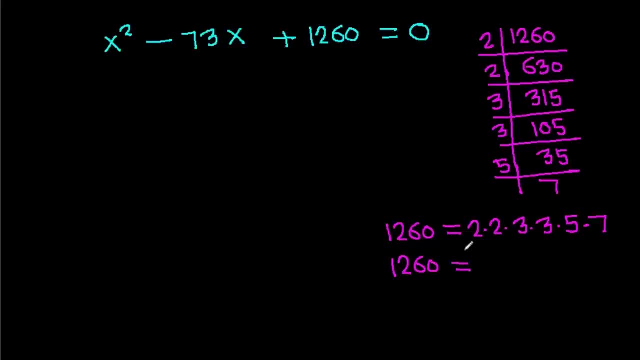 It is equal to: If we take 2,, 2 and 7 together, then 2 times 2 times 7 is 28 times 3 times 3 times 5 is 45. And 73. It is 28 plus 45.. 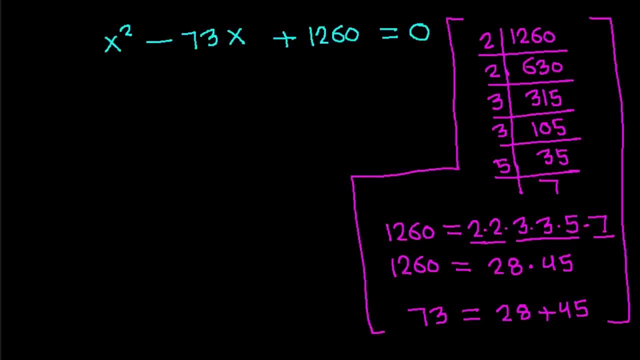 So it will be x square and minus 73x. It will be minus 28x minus 45x Plus 1260.. It is equal to 0.. And it is x times x minus 28 minus 45 times x minus 28.. 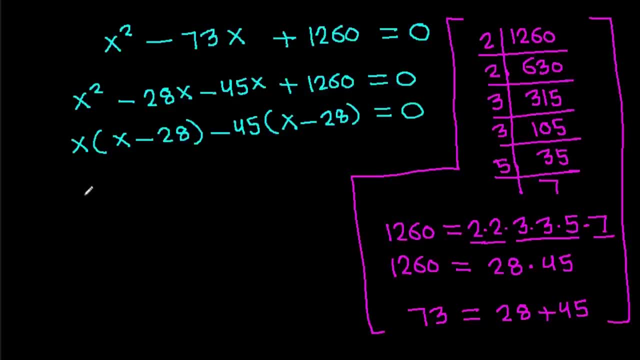 Is equal to 0. And it is x minus 45 times x minus 28 is equal to 0. So either x minus 45. It can be 0. So x will be equal to 45. And either x minus 28. It can be 0. So x will be equal to. 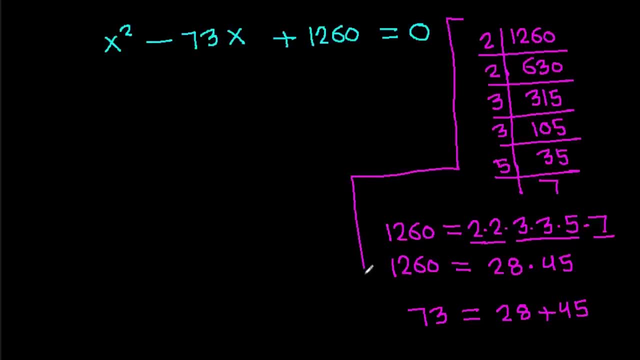 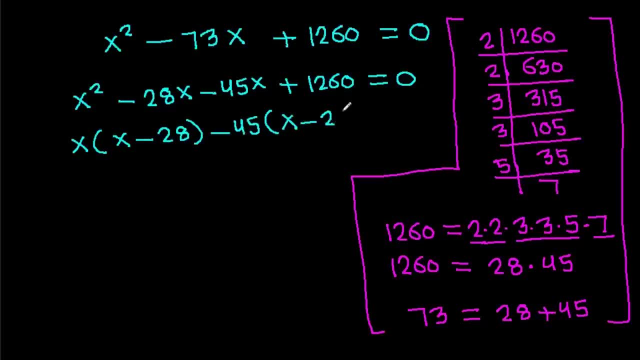 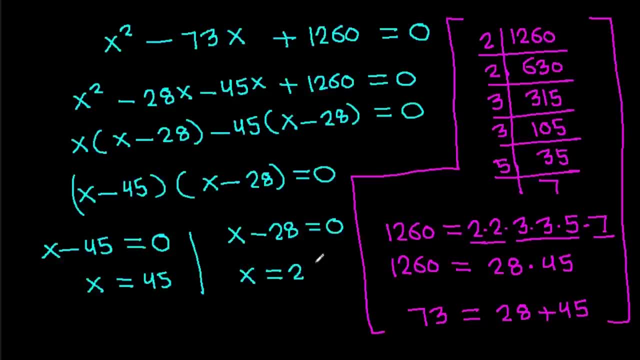 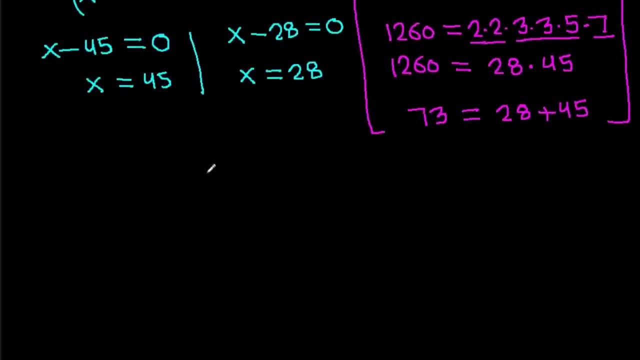 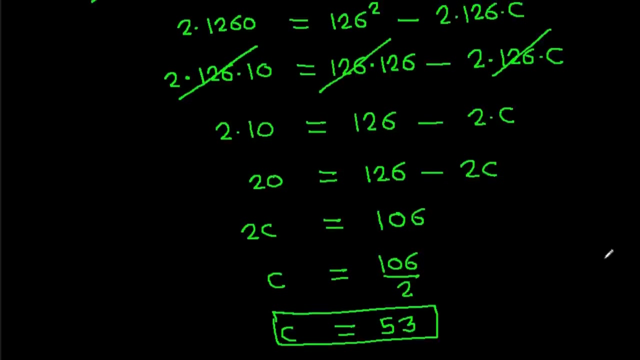 can be 0. So x will be equal to 28.. And we know that the root of this equation is a and b. So either a can be 45 and b can be 28, and either a can be 28 and b can be 45. And we have: c is 53. 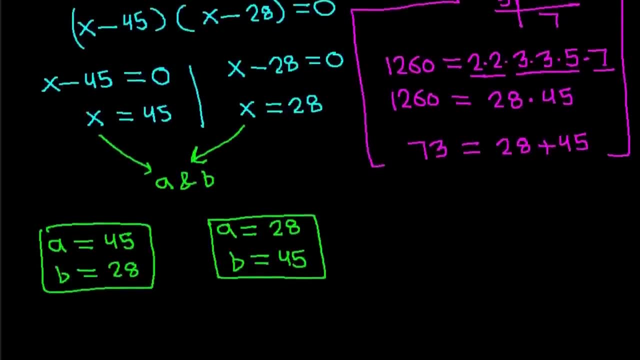 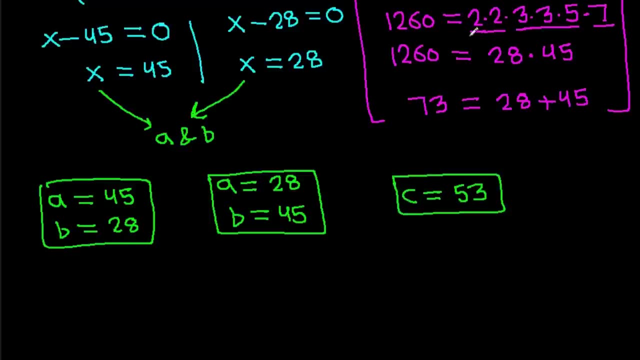 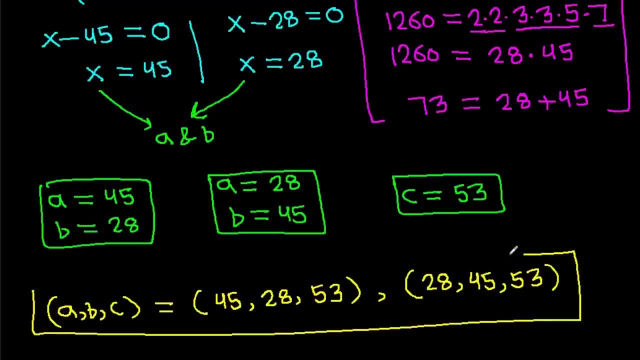 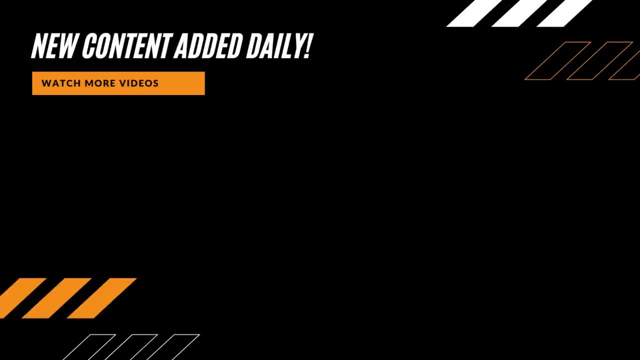 So a, b, c, it can be 45,, 28,, 53.. So a b, c, it can be 45,, 28,, 53..